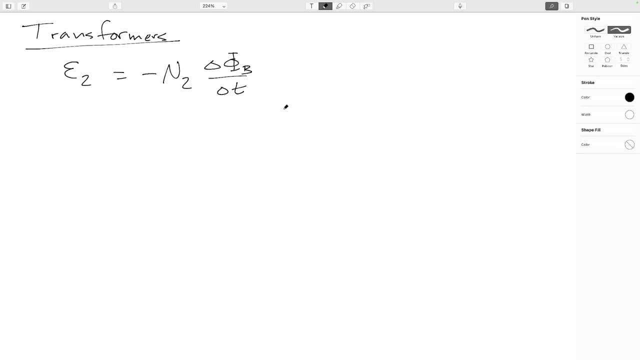 truly angle theictions of that coil. And here I grab the minus sign from the Maxwell equations, but it isn't going to matter because it's going to cancel out. Now what we can do is we can divide that by the input side, which is usually known as the primary, so primary one, and I can divide that. 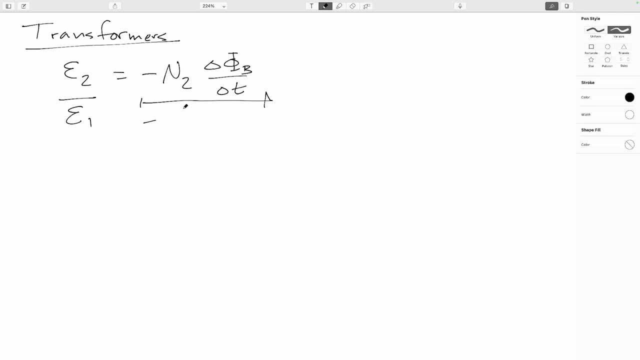 by the exact same expression We can. that will be equal to the number minus the number turns in the primary times the time rate of change of form. So I want to apply that equation here to work: four times rate of change of the magnetic flux through the primary. but since they share a common iron core, 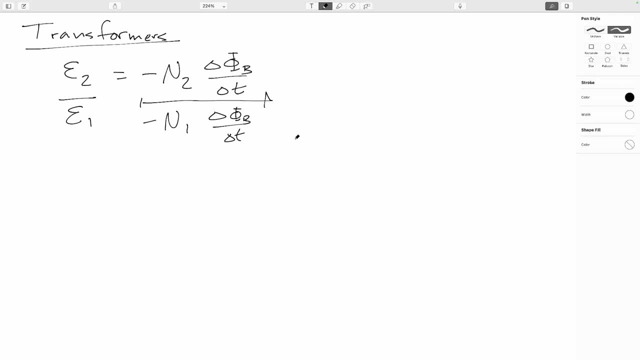 that means that the same magnetic field lines are going through both the primary and the secondary. that means that the, the change in flux through each of those is going to be identical, and so we can cancel them, and we can also cancel the minus signs. so this emf is going to be equal to the. 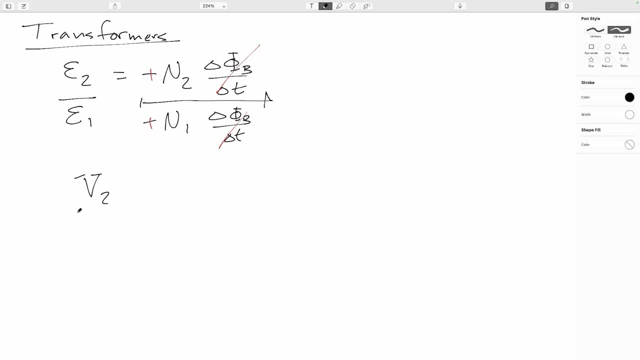 voltage across the secondary. so we can say the voltage, the ratio of the voltage across the secondary to the primary, will be equal to the number of churns in the secondary to the number of churns in the primary. so let's say that your primary had a, was a voltage of 120 volts. 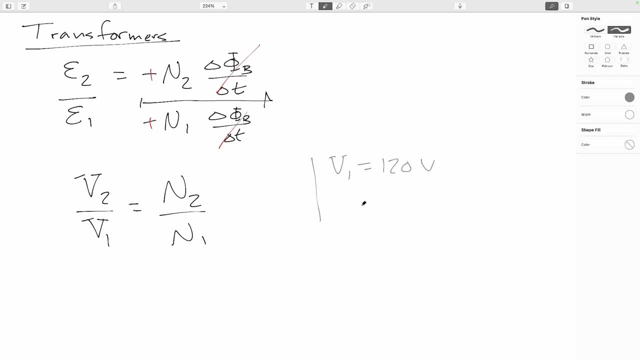 so we had 120 volts going into the transformer. let's say that you had um 2000 windings on the secondary and 200 windings on the primary. well, in this case here we could say that the voltage, if i multiply both sides by v1. 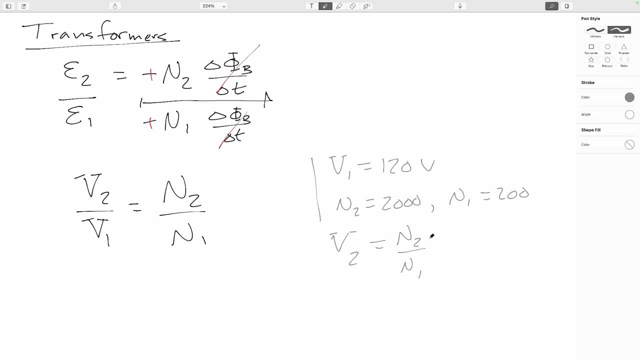 the voltage across the secondary will be n2 over n1 times the v1 um. this is going to be 2000 over 200 times 120 volts. well, this is a 10 to 1 ratio here. so the voltage across the secondary would be 1200 volts. so if i have 10 times as many turns on the secondary, 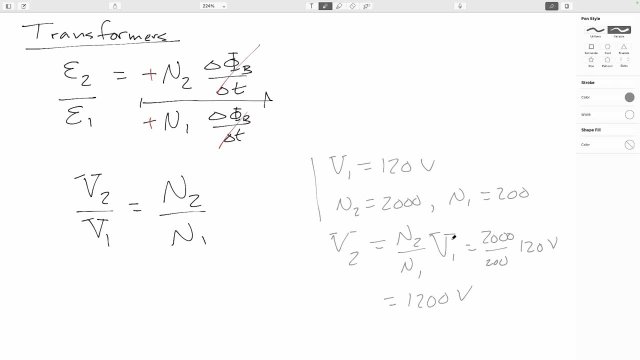 the voltage of the secondary will be 10 times. this is what we call a step up transformer. there's another definition of step-up, and whenever the voltage of the primary gets lower, this level in is squared. so pi divided by exponential zero is the size of the boundary. 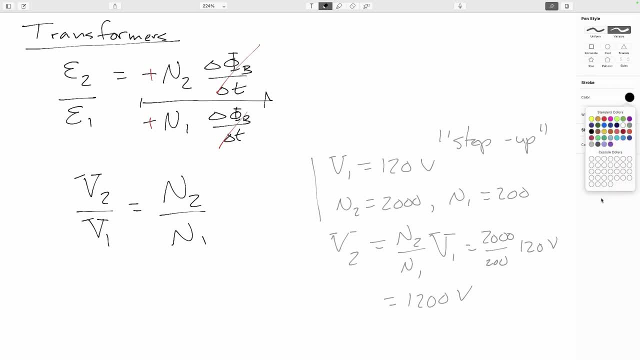 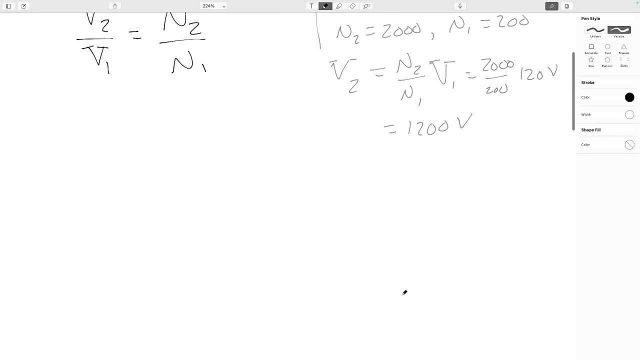 so already now we know that the output voltage is この. this is where the number of windings in the secondary is bigger than the number of wines in primary, so the output voltage of the secondary is higher than the input voltage on the primary. now you can't get something for nothing here and so 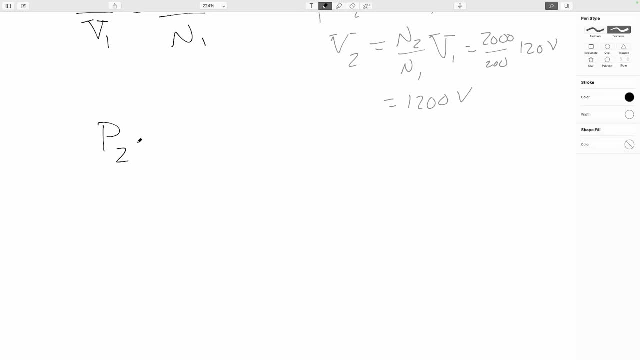 no, turned out that the um at which energy is being taken out of the secondary, that has to be equal to what was going into the primary. so that's, the power delivered by the secondary has to be equal to the power going into the primary. Well, the power. 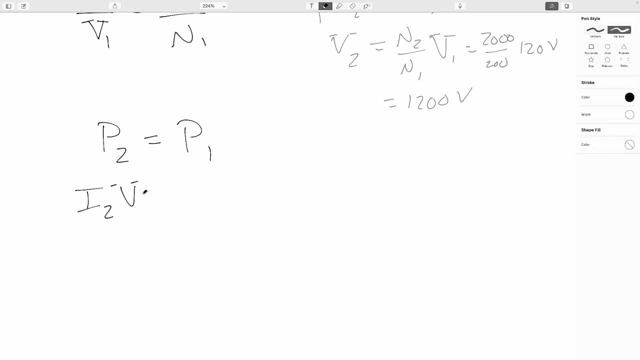 going into the secondary will be the current times, the voltage, and that's true for the primary as well. So we'll get that. so we'll get that I2 over I1,. the ratio of the current in the secondary to the primary is the ratio of. 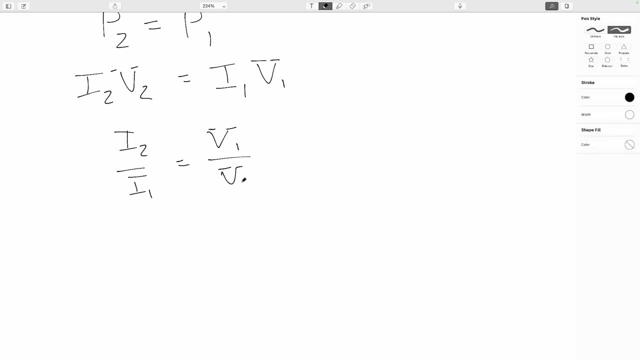 the voltage of the primary to the secondary, so the inverse ratio, And we just saw that that would have to be equal to the ratio of the primary number of turns in the primary to the number of turns in the secondary. So in our continuing our example, if I had 120 volt, 120 volts and 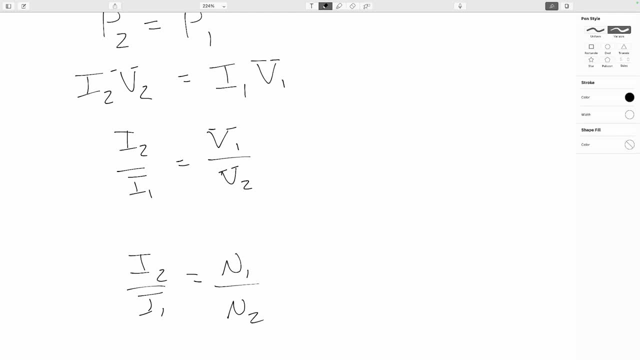 let's say one amp going into the primary, the voltage goes up by a factor of 10 to 1,200 volts and if I had one amp going, if I had one amp going into the primary, It's now a tenth of an amp. Now, where this is really useful practically is for the utility. 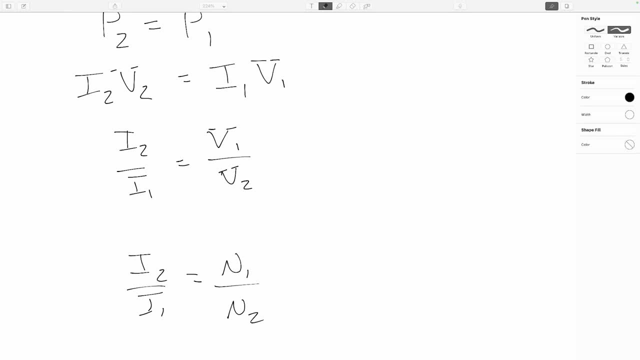 company. They're worried about power losses in the transmission lines themselves, And we remember that heat dissipated by any resistive anything is. I squared R. Now the resistivity of a power transmission line is kind of low, but the length of the power line is really long, And so this is. 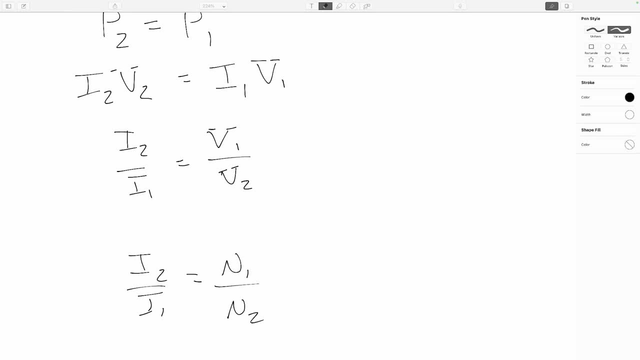 actually something that matters. So if I can drop the current by a factor of 10, because the losses in the transmission lines will go as the square of the current- that will give me a drop of a factor of 100 in the heat loss on the transmission lines. 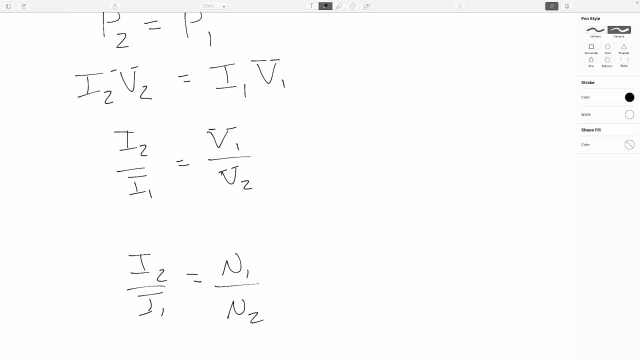 And the utility companies are usually doing much more than a 10 to 1 step up here. Now there are inefficiencies in using the transformer. You'll have step up on one side and you'll have to have step down transformers on the other side to get to more usable voltages. But even though there's losses, there's inefficiencies in the transformers. in each step of using transformer it turns out that those losses are exceptional. It's very susceptible, when weighed up against the savings, of how much energy you would be losing in the transmission line. 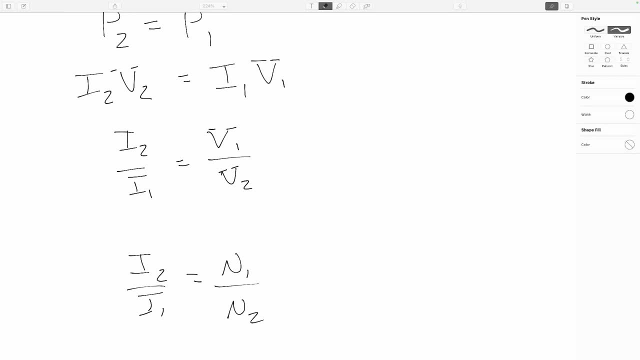 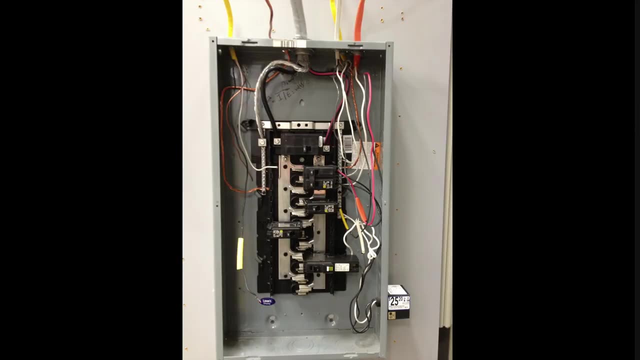 So with that, let's think about how power gets to your house, And we'll start by kind of working backwards here. So this is a typical North American circuit breaker panel, And I will be focusing on what happens in North America, where we use what's called split phase power distribution to residential areas. 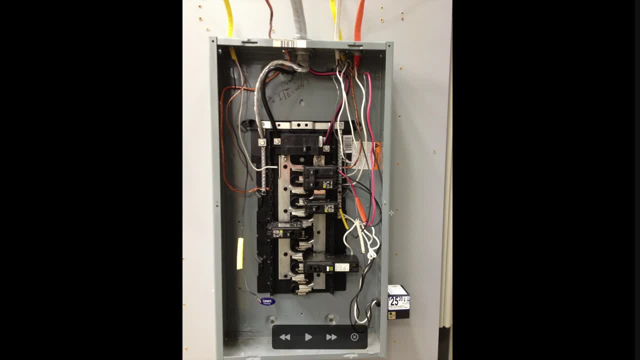 so going into you. so if you remove the protective metal cover in front of your breaker panel, this is what's behind it, this big cable. here is what's coming into your power mass from your power mast. this coiled a bit of braided wire. here is what's called the neutral. 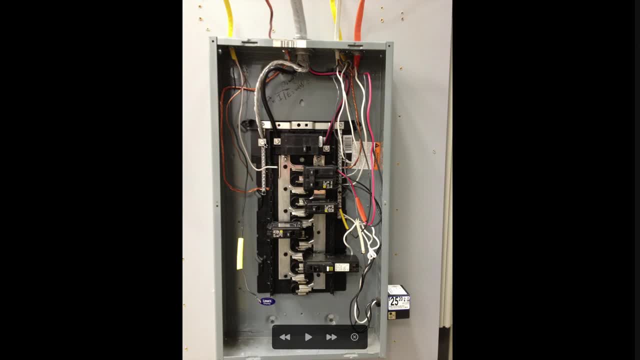 this could also be a white wire. it should stay at zero volts. in practice it might drift a little bit off of that. this black wire and this red wire are both what are called hot wires. this one is known as phase a and this one is known as phase b. 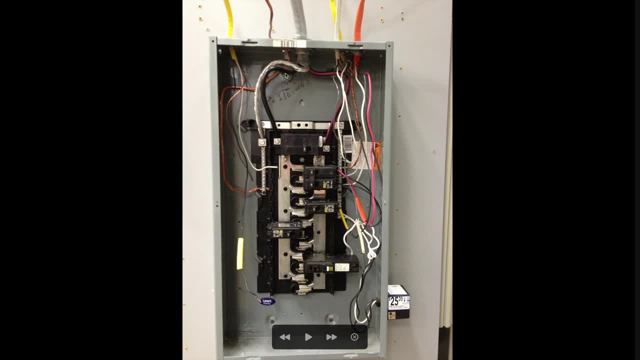 so remember: 120 volts ac means that you are oscillating between plus and minus 170 volts. so in phase a this is oscillating between plus 170 and minus 170, and so is phase b. however, they are 180 degrees out of phase. so when the voltage occur from between the black wire and the in the neutral 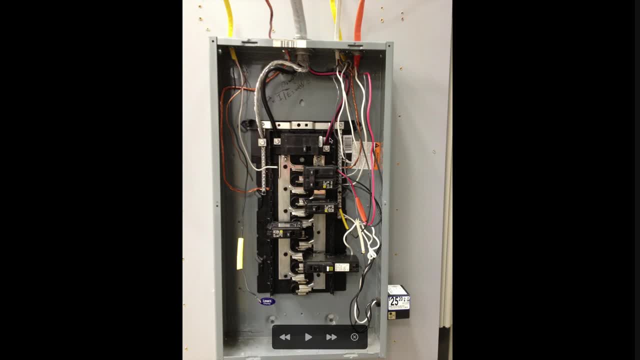 is plus 170 volts between the red wire and the neutral is minus 170 volts. so the difference is actually 340 volts maximum or 240 volts rms. so actually a potential difference of 240 volts is delivered into the house. now this big thing. here is the master breaker. if the current exceeds, 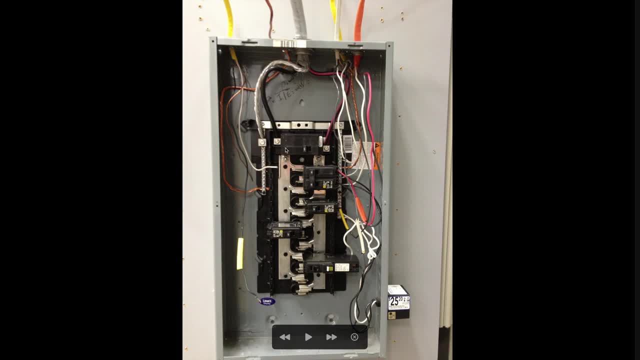 whatever it's rated for, in this case 100 amps, the master breaker will disconnect both phases from the entire house. now, going from there, the phase a exits the master breaker and goes on to this bus bar, and phase b also exits the master breaker and goes on to this bus bar here. 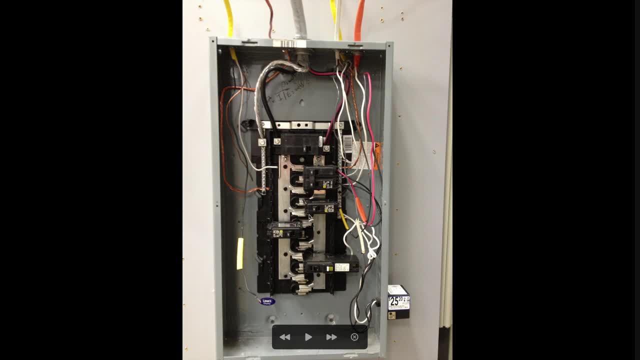 now you'll notice these little fingers coming out of the bus bar. this is so that you can have both 120 and 240 volt service in the house. so for the 120 volt devices, which is pretty much everything except your oven and your dryer and your air conditioner, 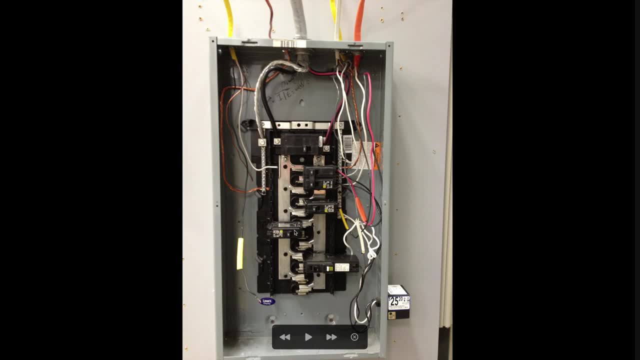 and possibly in your hot water heater if you, if you have that as electric um the this you can see here. this is just sitting on one bus bar. so if the and then the uh, and you can see a connection is brought off from one of these 120 volt breakers um to head off to provide service, along with a neutral. 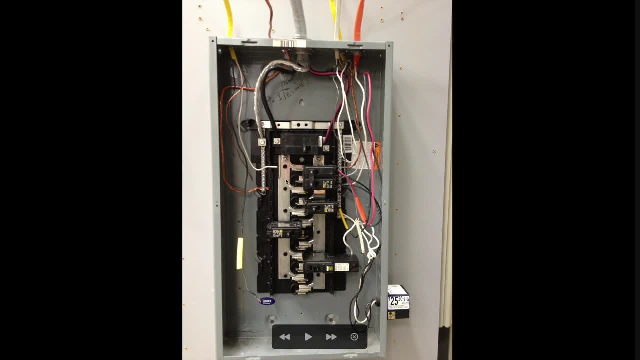 so if it's 120 volts you get either phase a or phase b and a neutral going through the romex and that connects off to the 120 volt outlets in your house. for the 240 volt service you send three wires: phase a, phase b and the neutral. now, in more modern houses there will also be 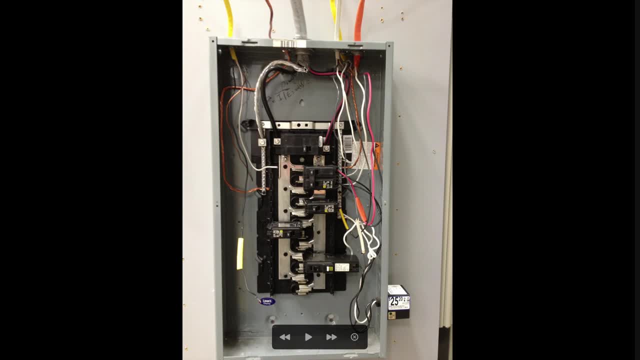 a separate ground. this is because, although the neutral should be at zero volts, it isn't always so. you can see the neutral is tied in on another bus bar here with a lot of screws and if you look right here, this screw is connected to a copper wire. 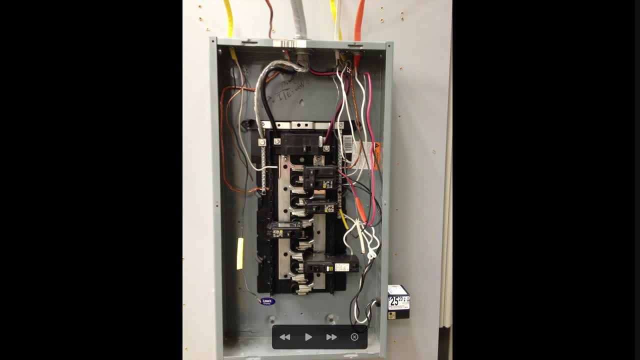 this copper wire would actually run, actually is going to run to the outside of the house, go underground and be attached to a couple of copper stakes buried under the ground. so the idea here is that the amount of charge on the earth at any given time is basically zero. 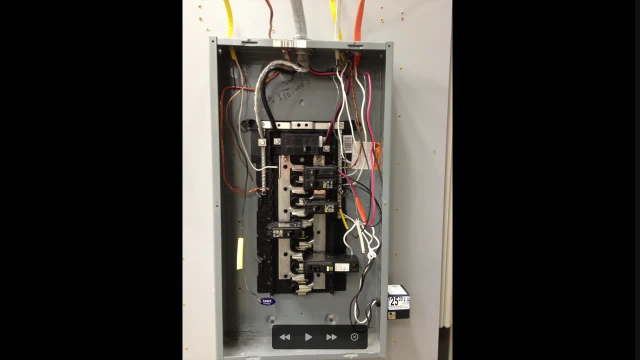 so we can just decide that the earth is zero volts and so this guarantees that the round prong, that the round prong as opposed to the blades in an outlet, are kept at zero volts all the time. the common that the neutral is tied to that, so it should also stay at zero volts, but there can be a. 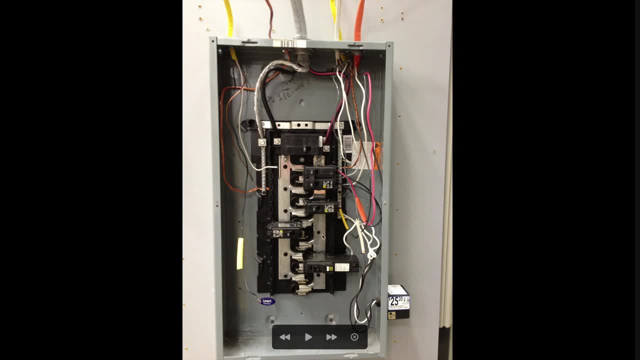 little bit of fluctuation because since you are pulling off of both phase a and phase b, the demand you know from one side of the house versus some other circuits in the house might not always be perfectly balanced and this can cause a little bit of drift. so whenever new circuits are added, electricians have to 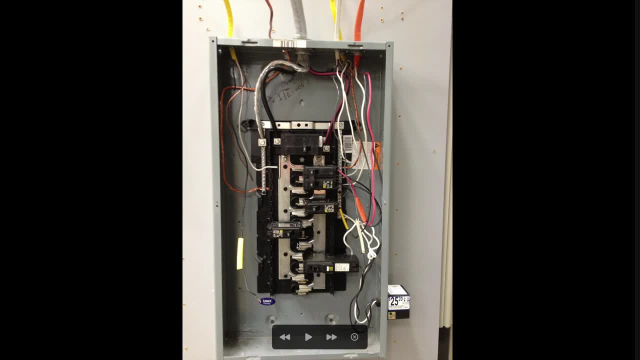 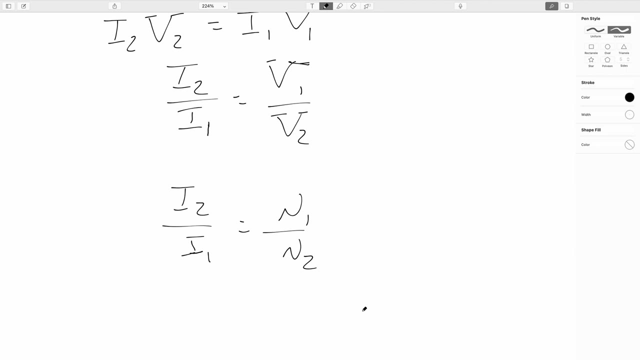 do calculations to figure out which side of the panel they should add the next circuit onto. so let's see what that looks like when it gets to the plugs in your house. so for the 120 volt plugs- so this is a 120 volt plug- you're going to have a wide blade and a narrow blade. 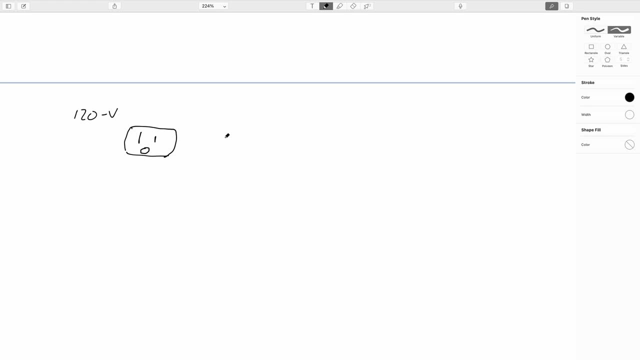 and around prong like so, and the short blade will be connected to what's called the hot- this is either phase a or phase b, but- and then the wider blade will be connected to the neutral, which should be zero volts, and then the round prong is the ground, which definitely is zero volts. 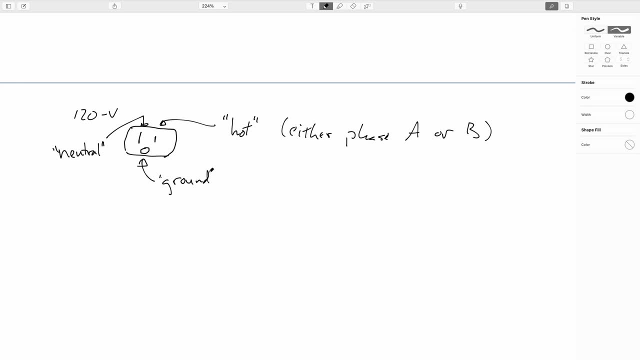 so that's a 120 volt outlet. um, if if it's looks like this, it means that the maximum that's this outlet can provide is 15 amps. if you see like a little t shape on one of these, then that means that you can provide up to 20 amps. 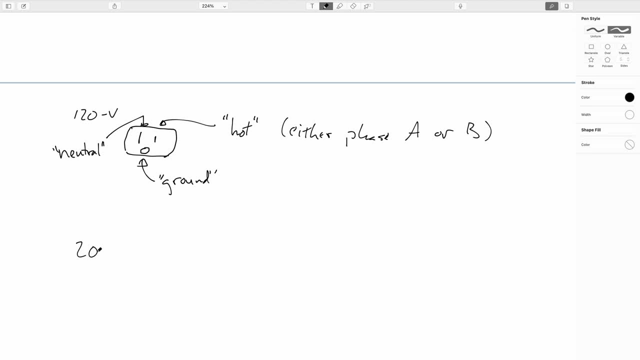 okay. so the problem here is that certain very high draw devices like your oven and your dryer can pull an awful lot of current, and so, again, the resistive losses within just the wires in the house can be so high that you run the very serious risk of catching the house on fire. 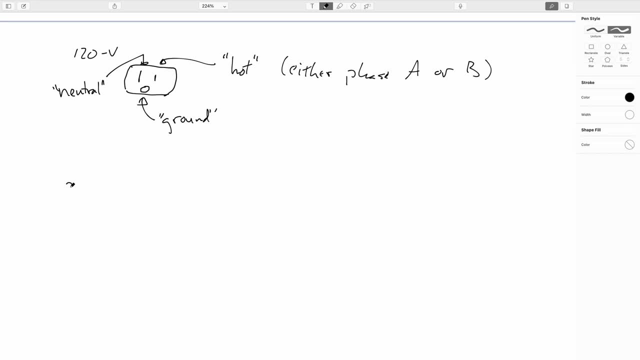 so this is where the 240 volt supply comes in. so your oven plug- which this is also used for recreational vehicles- will typically look something like this, and this is a much larger plug than the 120 volt plug. so you'll again have a round pin here, which is the ground. 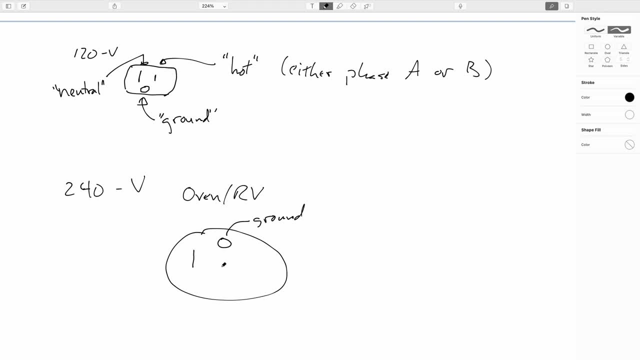 and you'll have three vertical blades like this. this one will. one of these will be phase a, um, so let's say it's that one. this one here will be phase b and then this one here is the neutral. so when you're running the oven, the cal rod in the oven is just connected directly. 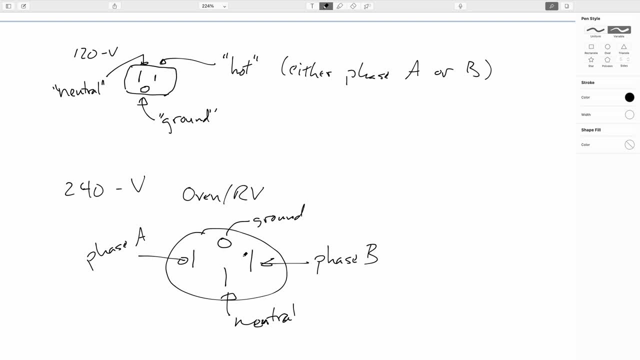 across phase a and phase b. so when this oscillates up to plus 170, this oscillates down to minus 170, for a grand total difference of 340 or 240 volts rms. by having double the voltage available, that means that the oven can pull half the current, which means that for the same size wire, the rate 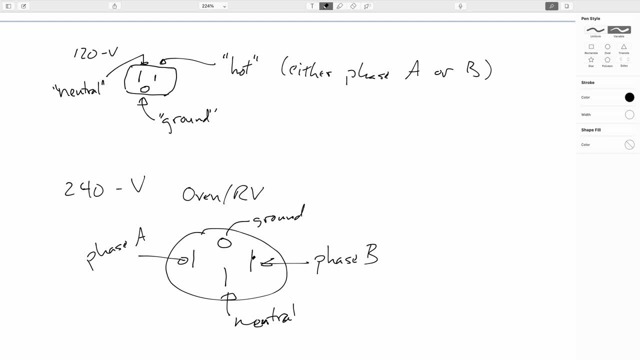 at which the wire leading to the oven is dissipating heat is dropped by a factor of four. this is enough to um make sure that you don't have to have fire hydrants in the oven. to make sure that you don't have to have fire hydrants in the oven. 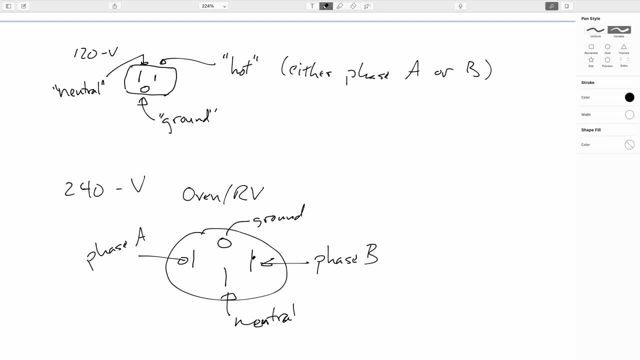 for your host sized wires. okay, i'm exaggerating a bit, but very this means that you don't have to have very, very fat wires in order to keep the heat losses under control, um, your, your dryer, um. so this is designed to pull a maximum of 50 amps. 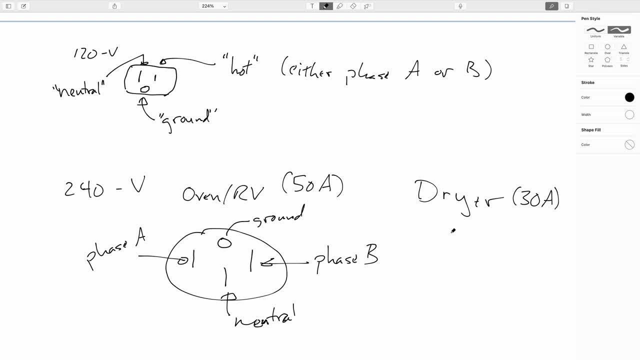 your dryer is designed to pull a maximum of 50 amps. the dryer is typically rated for 30 amps and the pin and the plug looks basically the same. um, this is still ground. this is still phase a. this is still phase b. the difference is the neutral. the blade for the neutral is kind of bent into an 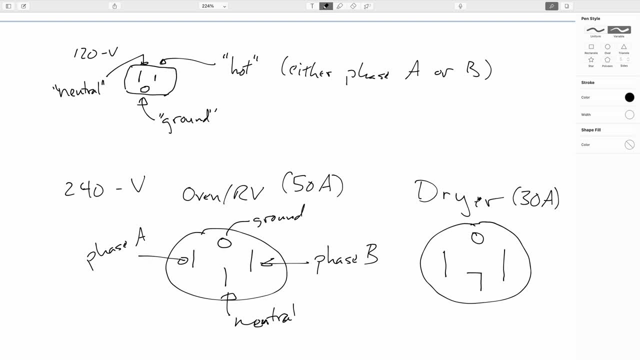 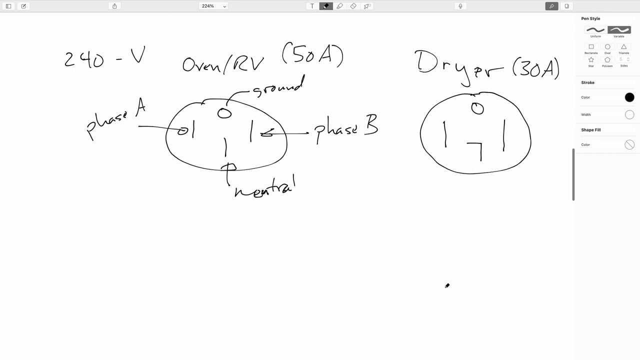 l shape like that, and this is just to make sure that you don't plug your oven into a dryer outlet, because that could be bad. but again, it's the same layout: phase a, phase b, neutral. now these are the more modern designs, so this will be for construction. since the late 1980s, older designs did not have. 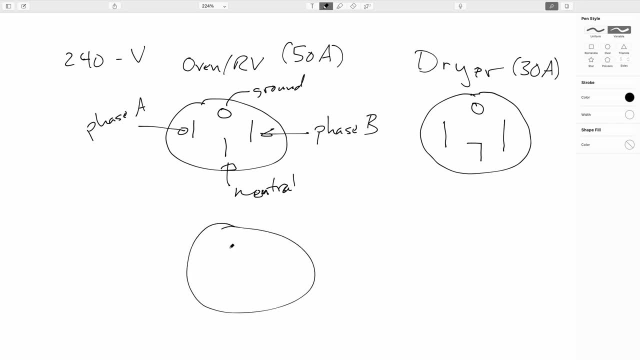 the third prong ground, and so they would have looked like this and like that, and the idea was that, well, of course the com, the neutral, should be at zero um, so we'll just assume it is. but here's the thing: the way that the, so the dryer um sends phase a, connects the 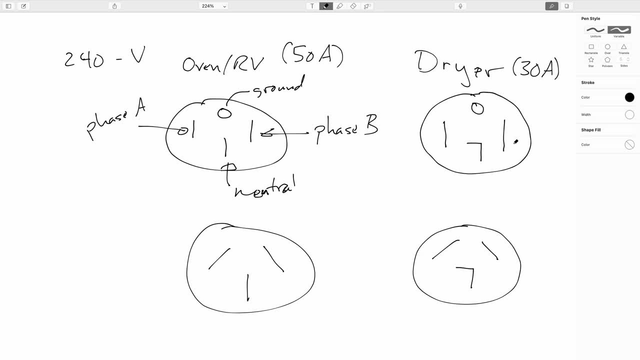 heating element across phase a and phase b, but the motor in the dryer is probably 120 volt motor and so they would just connect the neutral to one of the phases because this is staying at basically zero. well, this means that you're pulling slightly more current from one than the other, and this will cause a bit of a drift in. 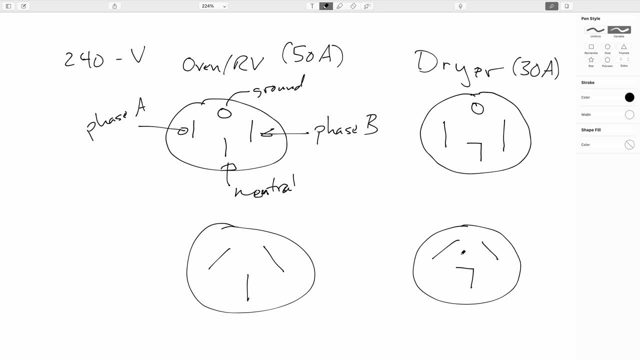 the voltage here. so if you're down in the basement and also the ground, the chassis- for safety reasons- is um attached to the ground. so here you're making the assumption that it was grounded, but the voltage was actually drifting a little bit and in a basement, in a laundry, you could very well have. 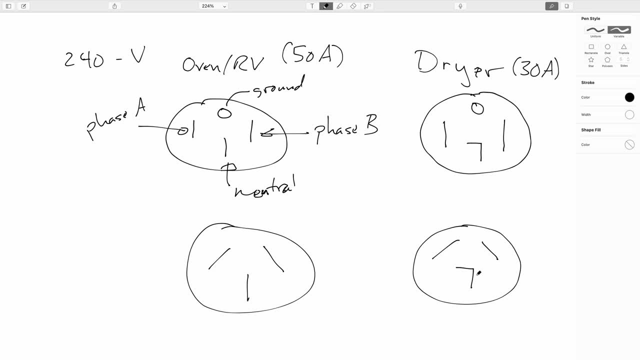 a wet floor and if you're standing there with in bare feet in a puddle that was caused by you doing laundry not very well, um, and then you touch the dryer while it was running there, it could be the case that the chassis of the ground which is hooked up to this pin could actually be at a few volts. 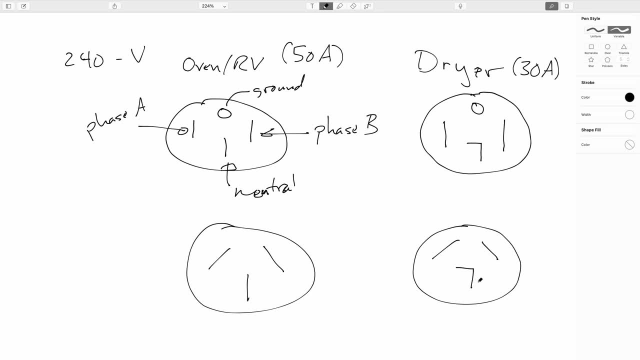 and you get a little bit of a zap, and that wasn't a good thing. so, generally speaking, the ground is guaranteed to be at zero volts, and so if you touch the dryer while you're standing in a puddle, the ground, which is guaranteed to be at zero, came in and now the chassis of the dryer is attached. 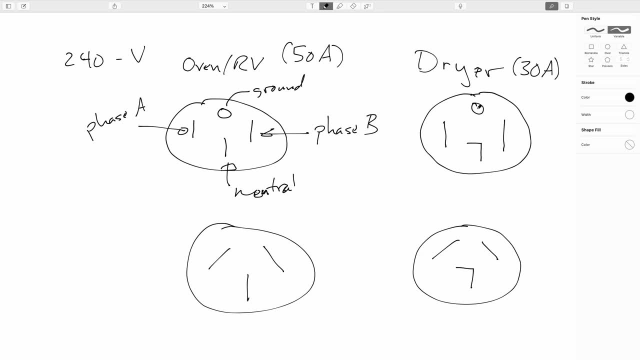 to this pin here. so then, if you touch it while standing in a puddle, you really shouldn't, but if you do it accidentally, this is guaranteed to be at zero volts. the puddle that you're standing in will find you a pathway to ground which is also zero volts, and so you won't pull any. 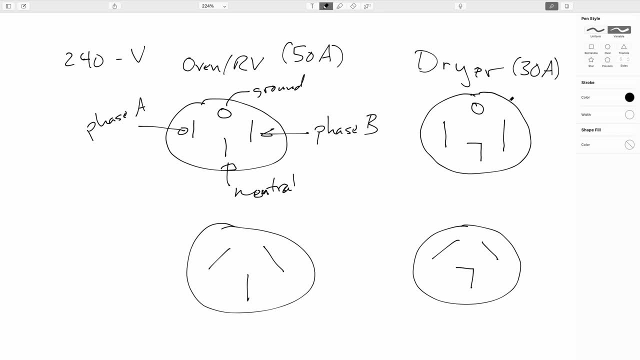 current through you, and you won't get a surprise. now, how does it get from? how does it get to your house? well, it turns out that the way power is delivered up to the neighborhood is a thing called three-phase transmission, which i won't really get into too much here. 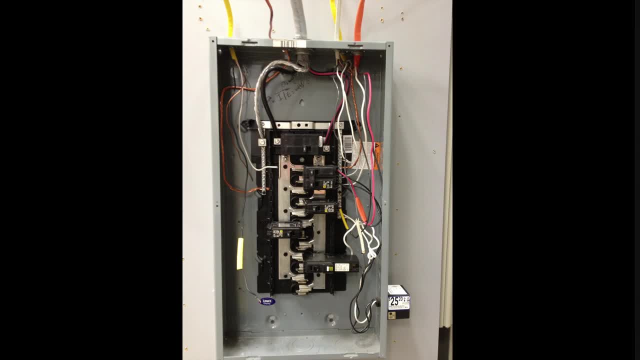 suffice it to say three-phase is what they use in europe and three-phase is delivered straight to the house and there are a lot of advantages to it. but for historic reasons we've got this. but three-phase is delivered straight to the factory because you can build nicer motors with. 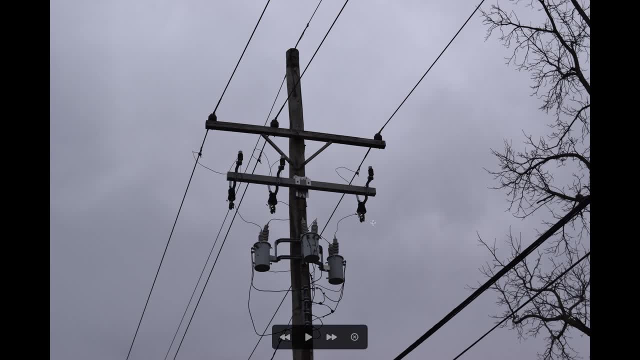 three-phase. so anyway, within a few kilometers of your house, you're probably going to see on a utility pole something that looks like this: this is where they are pulling out the three-phase that's coming. the three phases are coming from the substation and they're sending phases to 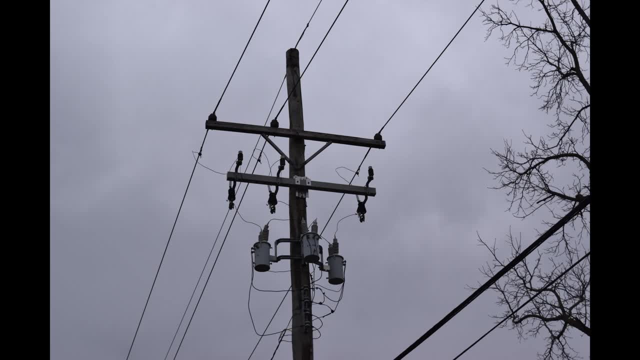 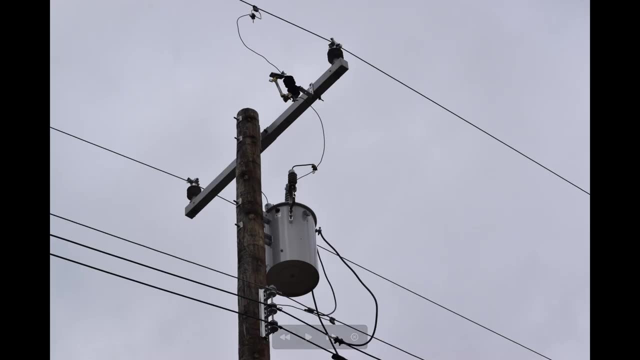 individual phases to different neighborhoods in in the area. when you so coming in here, what you've got is: you can see this is a transformer here. this is attached to one of the phases coming in from the power company and this is at a depends on the power company and how they're doing it, but typically, 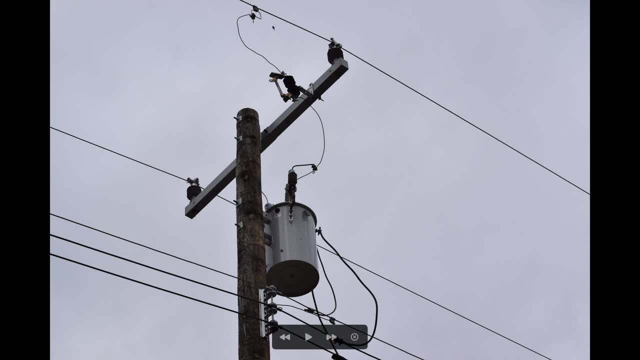 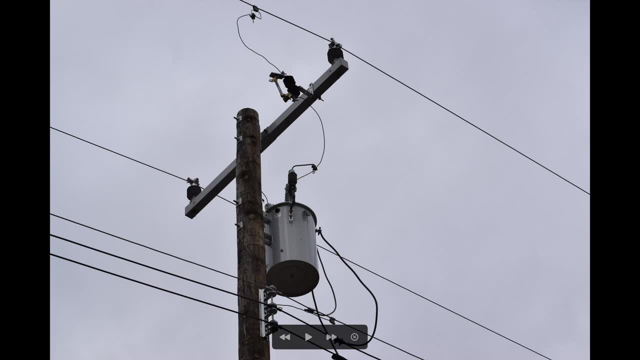 along on one side and then a earth ground line onto the other side to a transformer that's in this can. also in this can is a really big honking fuse, just in case things go really bad. um, now, if you are lucky enough to be somewhere where they actually bury the power lines, 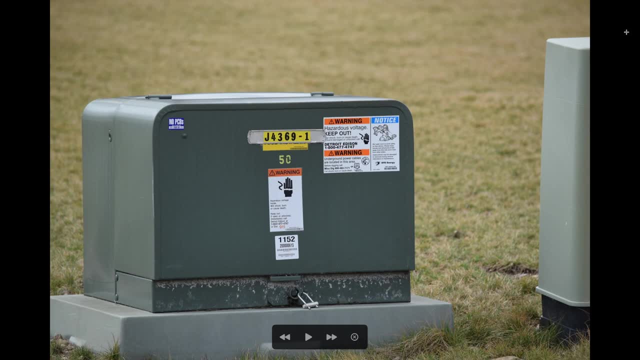 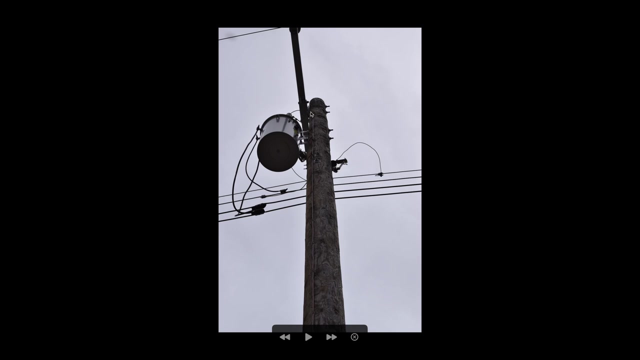 that will be sitting in, typically a green box that looks something like this, but it's the same thing, it's just you can't see the wires. so anyway, we can see here that the there's a wire coming in from one of the phases being provided, goes into the transformer and you can see coming out of the transformer are three leads going to. 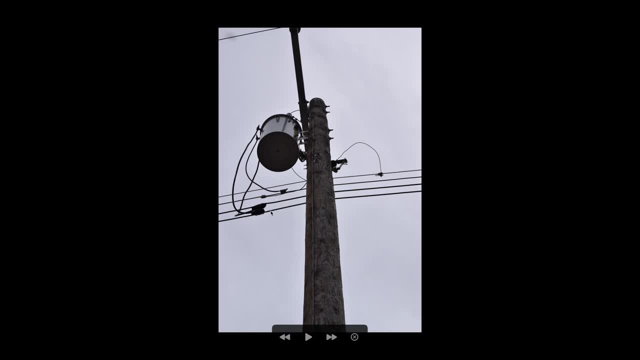 three wires. one of these is phase a, one of these is phase b and the other is our neutral. so how do we achieve that? well, see, this wire is going to be in the transformer and the other is going to be in the wire going down here. first off, that's the earth ground for one side of the power transmission. 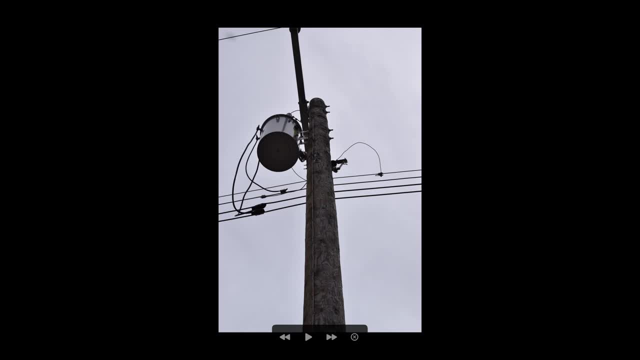 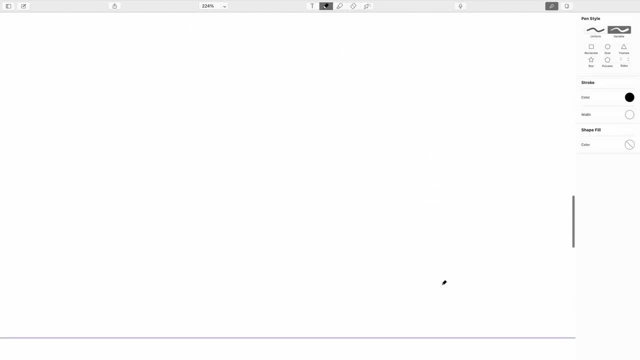 but also coming out of the transformer. transformer is wired up something. it's hooked up something like this: so this is the symbol for a transformer. so these are the two coils in the transformer. let's say this one's the primary and this one is the secondary. um, this pair of lines here means that it's just a magnetic connection. there's no electrical. 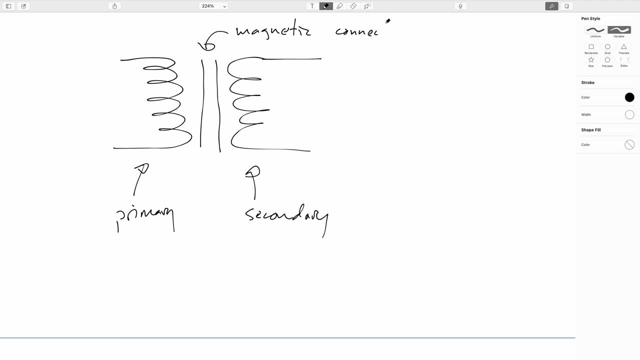 connection. so these two coils share a common magnetic field. so what they do is the primary comes in at about 7 000 volts ish um and then gets stepped down to about 240 volts. if you notice, the wires going in into the transformer are much thinner than the. 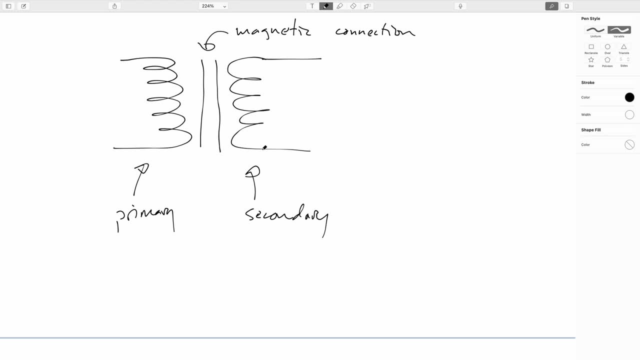 ones going out. this is because the wires are much thinner than the ones going out, because when we step down the voltage we step up the current, so we have to make the wires fatter in order to reduce transmission losses in the line. but then what they do to provide the split phase? 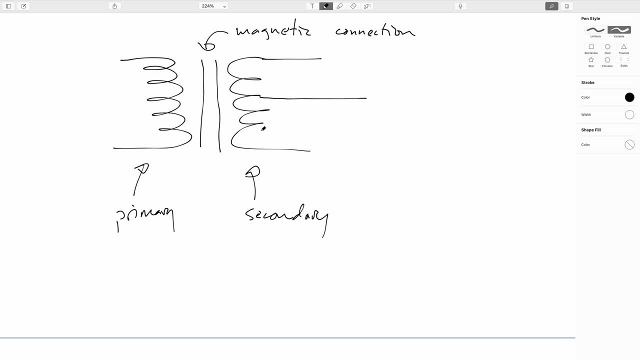 is that there's actually a third connection just tied in somewhere in the middle of the coil, actually at the exact center of the coil, and then this is what gets run down that wire, down the post, going all the way down the wire and then going all the way down the wire and then going all the way down the wire. 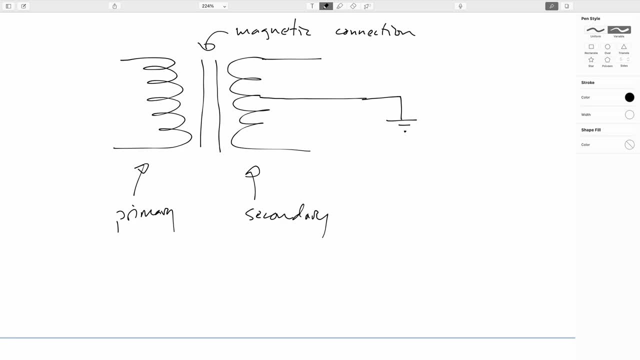 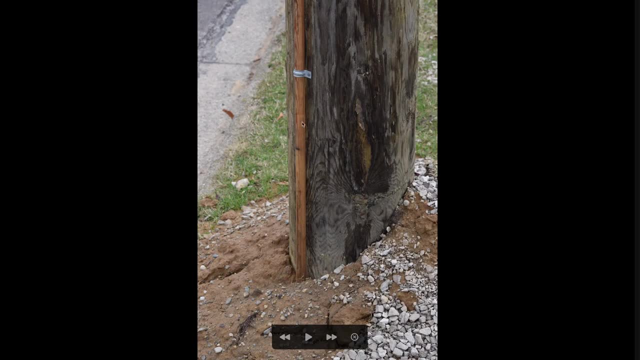 way into a stake in the earth. There's a little cover here just to make sure people you know nobody cuts it accidentally or anything like that. but the wires continue to run down the pole and into a stake in the earth. So again, 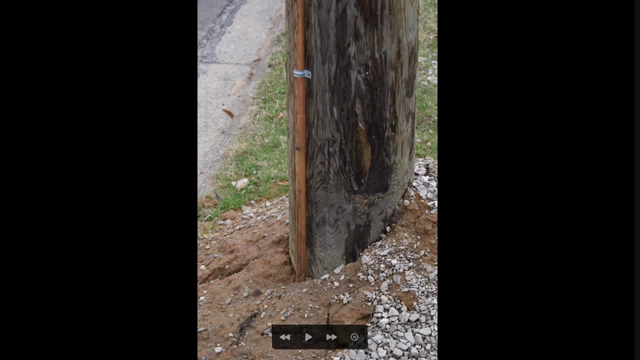 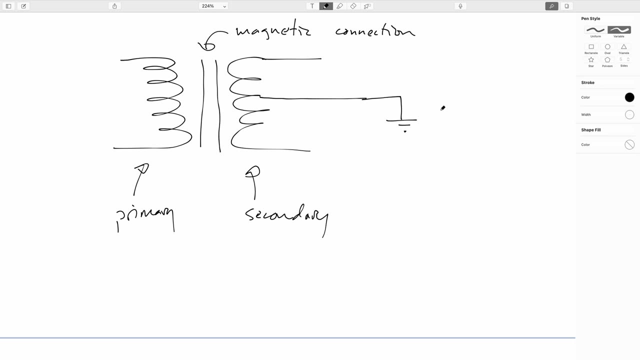 guaranteeing that it is at 0 volts. So the symbol for that is this: so that just means ground. So we've set this to be at 0 volts, but the difference across these is 240 volts, so that means that there is a 120 volt. 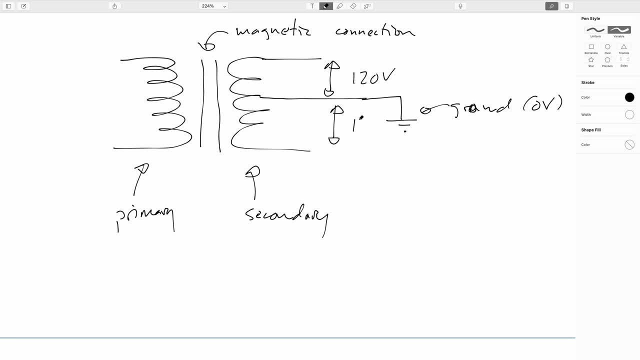 difference here- thanks for watching and I'll see you next time- and the 120-volt difference here, but the difference across the whole thing will be 240.. So this becomes your phase A and this becomes your phase B, going into the house. 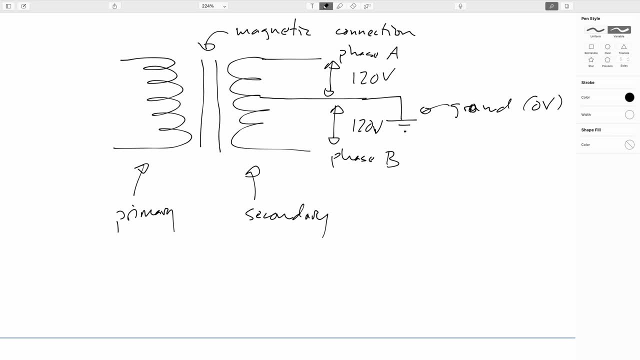 All right, but where did it come from there? 7,200 volts is still a really high voltage, and it's because they can't step it all the way down to 240 from the substation. The runs would be too long. So up to a few kilometers away probably from where you're at, from where these 7,200-volt lines are, you'll probably see. You'll probably see in high-tension lines like these, where these could be anywhere on the order of about a half a million volts. 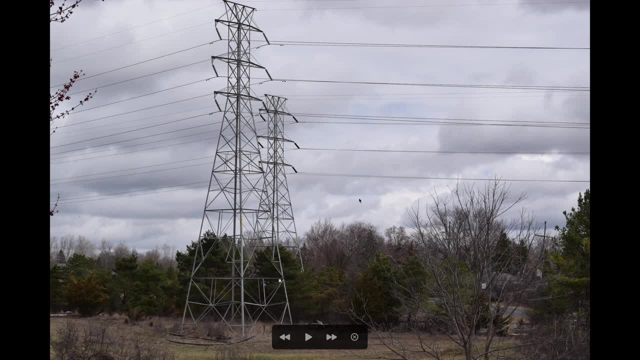 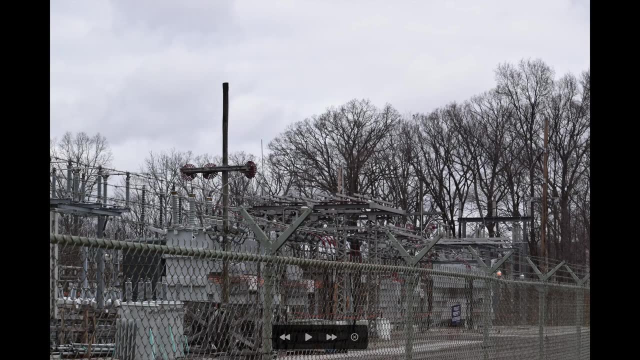 potential difference or even higher, And they will go into typically fenced-off installations like this, because, unless you know what you're doing- I mean all these wires that you see here- they're not insulated, They are at ridiculous voltages. 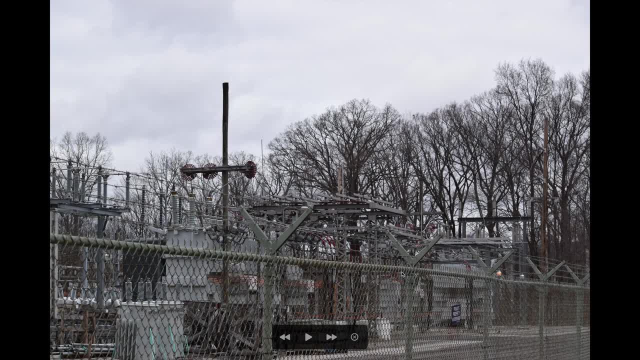 You touch one of those, not knowing what you're doing, you will fry yourself And you can see these huge boxes there. Yeah, those are transformers, like right there. They are really, really big transformers And they're stepping down from the half a million or so volts. 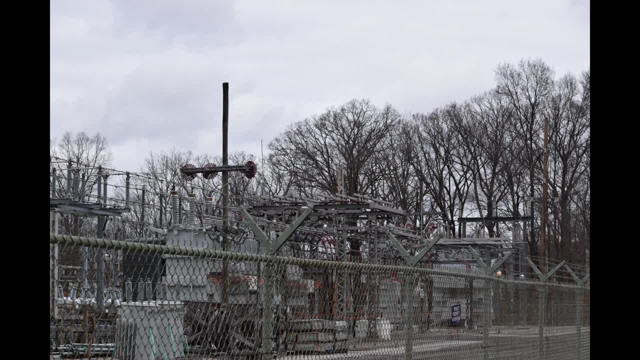 down to the 7,000 or so volts And the current going through the wires will go up in proportion. So, on the other end, when you have a power factory or power plant, typically they tend to produce electricity at about 10,000 volts or so. 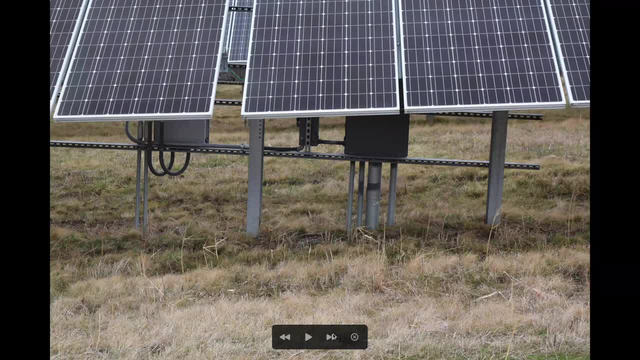 and then it goes and gets stepped up. So here's an example of a nice power factory here. This is taken from. This is taken from a solar farm. Now, solar panels are uniquely DC devices. However, there exists a device called an inverter. 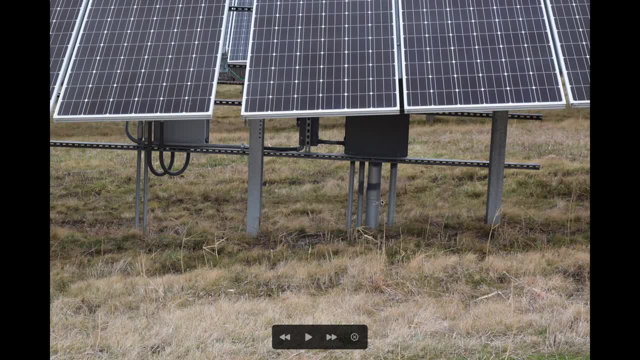 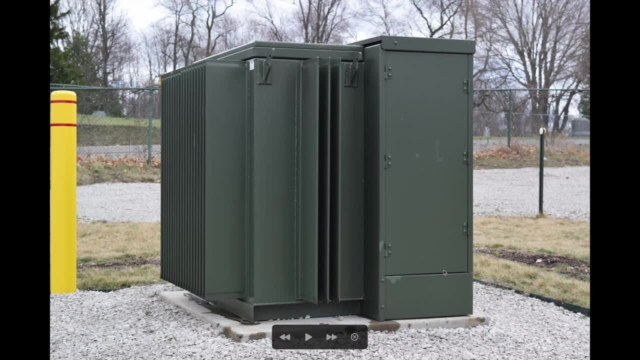 that will take DC and turn it into AC. The outputs from all these inverters are combined in a giant, basically power panel to make about a 600-volt AC connection in this particular power farm, And then this gets stepped up to- in this case, 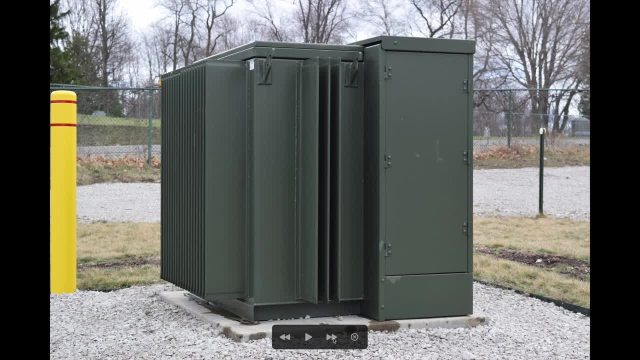 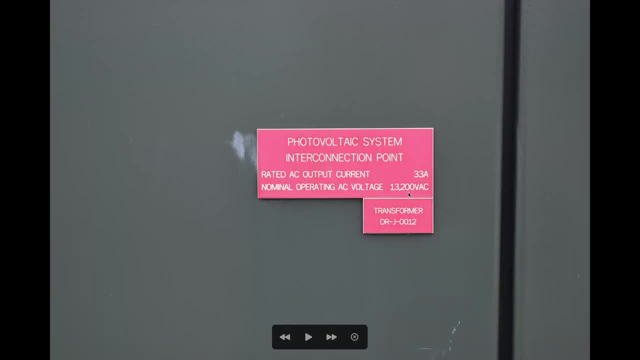 about 13,000 volts And this will find its way to some step-up transformer to go into the grid. Now take a look at this. So this is at 13,000 volts, The current going through the wires coming out of the transformer. 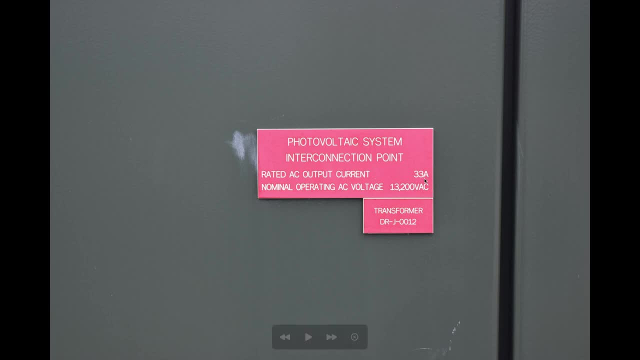 is a measly 33 amps, And yet this corresponds to over 400 kilowatts of power being delivered to the neighborhood. So with only 33 amps, the losses in the transmission lines are acceptable. Now things are changing a bit. I've already mentioned that solar panels are uniquely DC, And so there is some thought that with household power solar panels, especially if you also have battery storage, which is itself DC, that you might want to start running DC wiring from the solar panel into the battery. 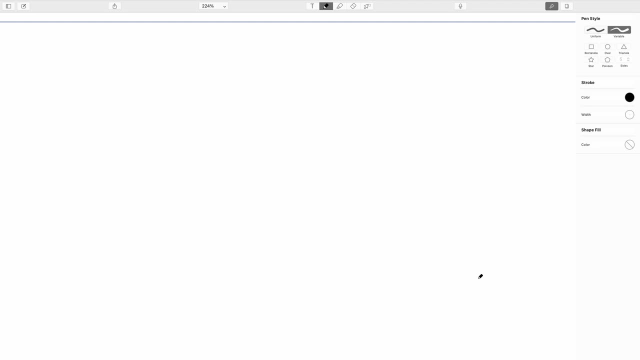 In fact, this is actually what's done in a lot of sailing vessels, And then you'll again use these inverters to get yourself AC for the rest of your devices in the house. The other thing where DC is starting to come back into play. 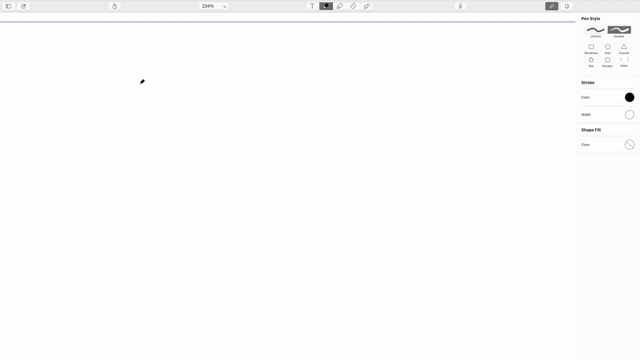 is. there is sort of a funny effect in AC If we look at a cross-section of wire. it turns out that in AC the closer you are to the outside of the wire, the greater the density effect. So if you look at the outside of the wire, 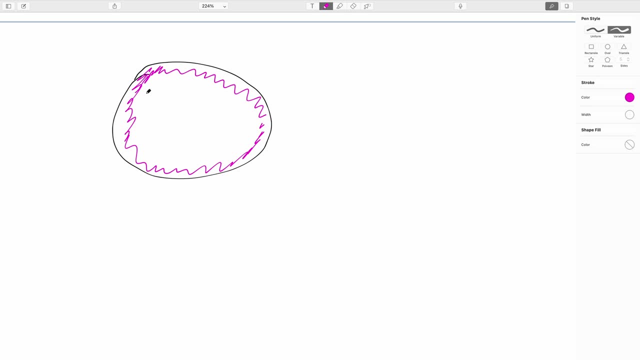 the greater the density of current that gets transmitted. So most of the current- this is an effect called skin depth. It's way beyond the scope of this presentation to get into what happens, But suffice it to say that the bulk of the current gets transmitted on the outside. 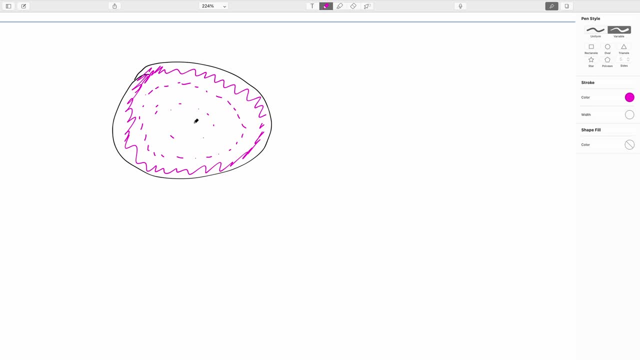 and the amount of current going through into the interior of the wire gets less and less and less Transmission lines. just remember: the bigger you make a wire, the less its resistance. Transmission lines use very, very big wires But, however, since you're only basically using the outside of it, 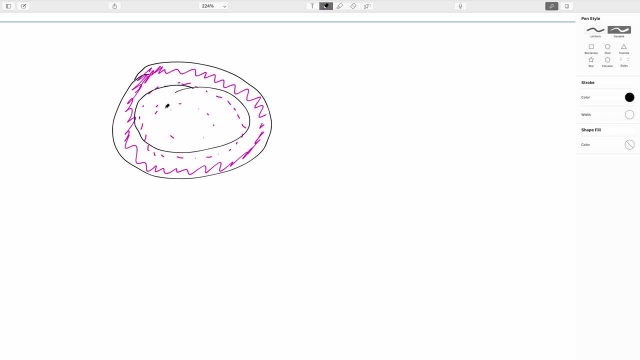 most transmission lines are actually hollow. There are spacers stuck inside so that, since you're only using this much of it, you need to leave it hollow to save some electricity, Save some cost- A lot of cost actually. But this: it turns out that trying to do runs 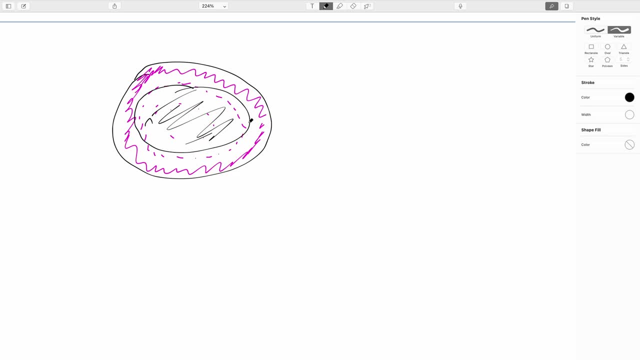 of more than, like, say, 1,000 kilometers or so, even at half a million million volts, the losses become unacceptable. Then someone came up with a clever trick. There is a DC, there is a device called AC. 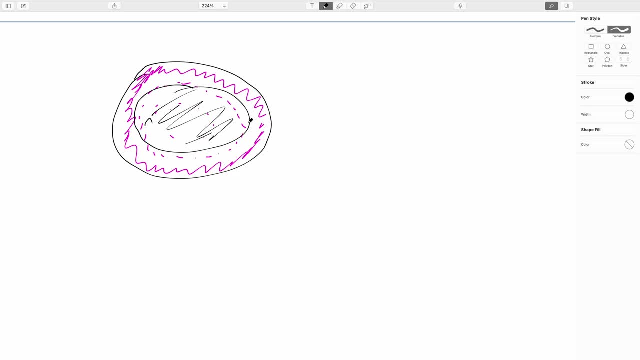 and a rectifier that will take AC and turn it into DC And so kind of in a funny circle. in areas where very long runs are needed for the grid, like, say, interconnects between, say, Scotland and continental Europe, is one example. There are a few others that are going back to DC. This is because with DC, the current is uniformly transmitted through the wire. So although it's a fatter, so you can use a fatter wire. but not only that, since it's distributed uniformly. 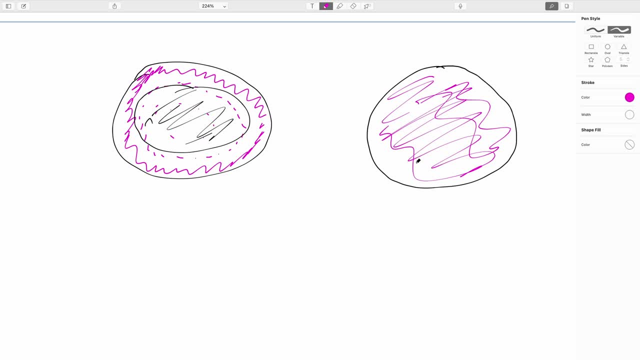 you can deliver a lot more current through. The trick was being able to make DC inverters that would allow you to go up to a million volts. So again, very low currents going, comparatively speaking, going through these very, very fat wires.